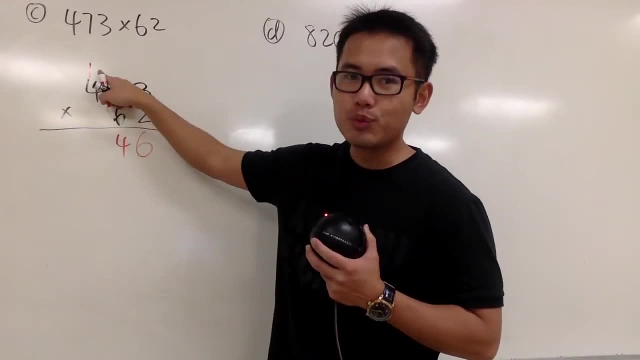 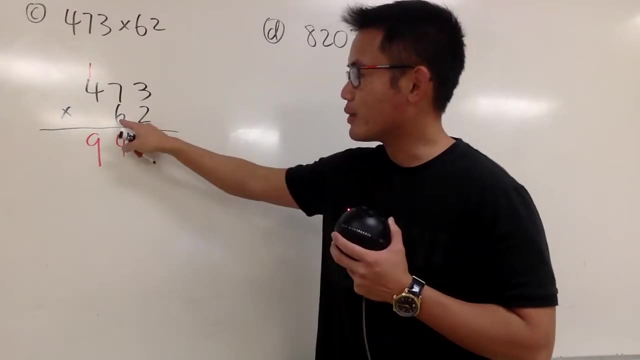 And then 2 times 4 is 8, but we have this 1, right. 8 plus 1, we get 9.. So this is it, And now we are going to move on to the 6.. 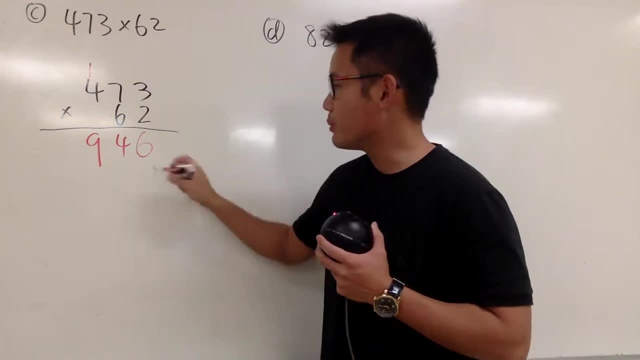 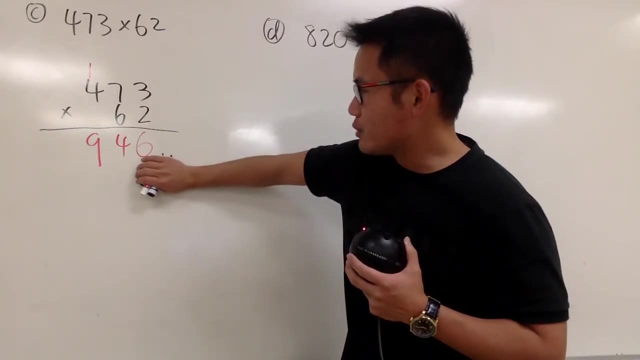 And it's going to be right here for the second row right And be sure you put down a 0 right here before you continue. Some teachers will tell you to put down x, but you just have to remember this. right here is not where you are going to start. 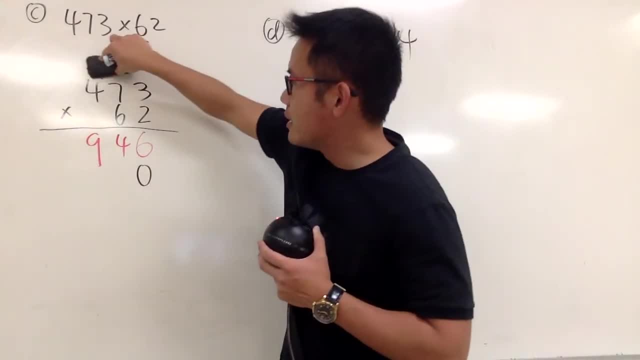 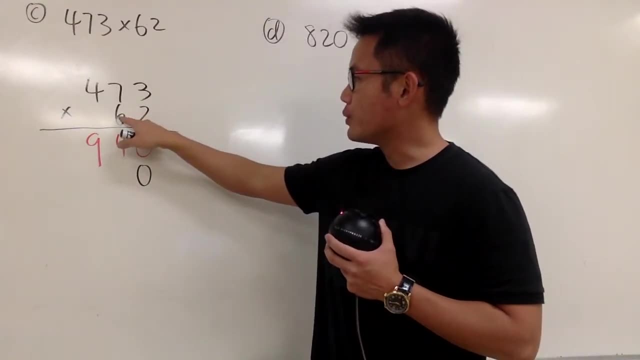 So it's the answer: stay strong. And I'm going to erase the 1, because that was for the 2 earlier, right. 2 times 7 was 14.. Now we are going to do 6 times 3,, which is 18, right. 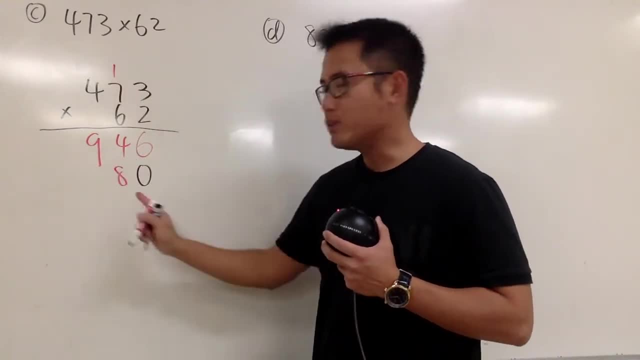 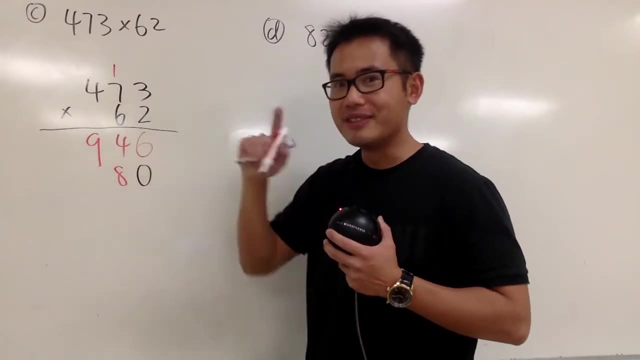 I will put down 1, 8, like this, And you see, we put down the 8 right here to begin with, right, And now 6 times 4,, I mean 6 times 7 is 42.. 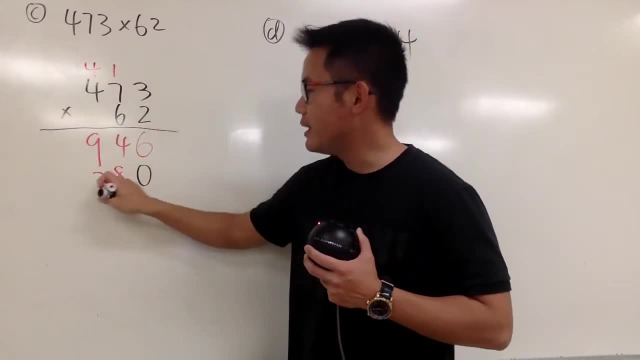 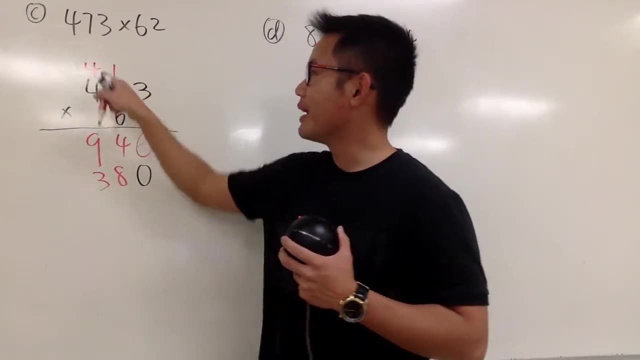 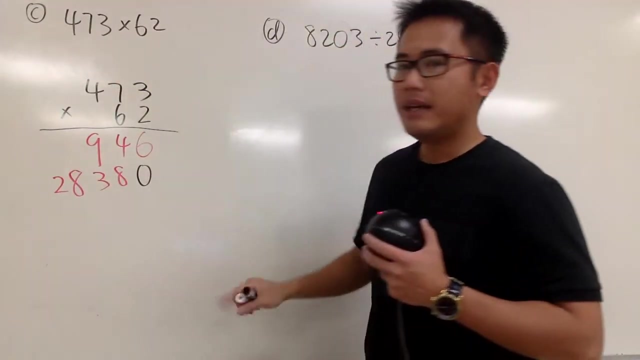 42 plus 1 is 43. Like that, right, 43.. Lastly, 6 times 4 is 24, plus this 4,, we get 28,. okay, So this is how you finish all that, And in the end, we are just going to add them up. 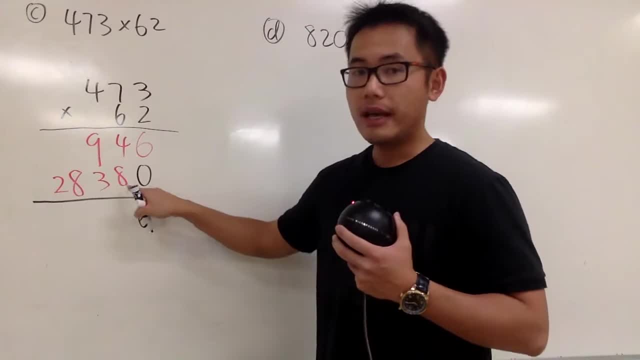 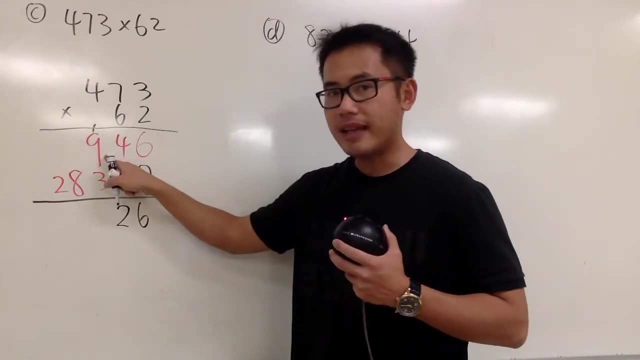 So now 6 plus 0 is 6.. 4 plus 8 is 12.. So I'll put down 1, 2 like this, So 1, 2.. And then 1 plus 9 is 10.. 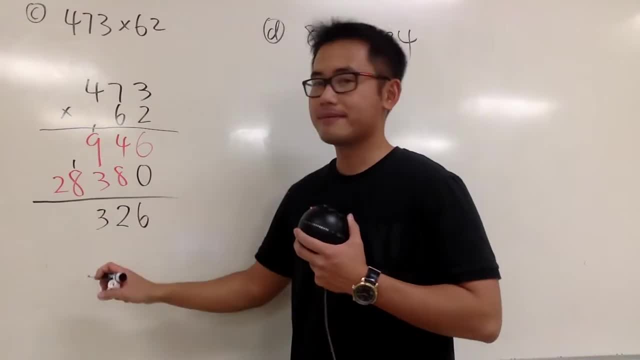 10 plus 3 is 13.. So we have the 1,- 3. Right, And then 1 plus 8 is 9.. And then, lastly, we have the 2.. So final answer. 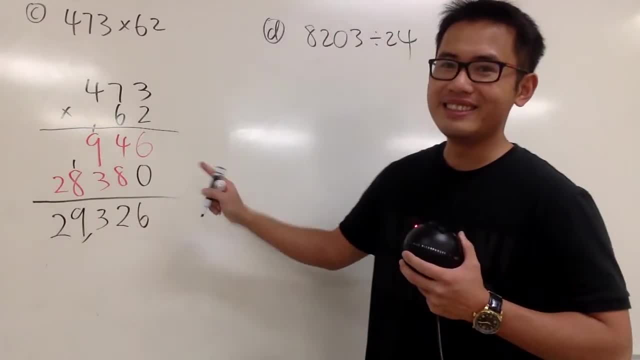 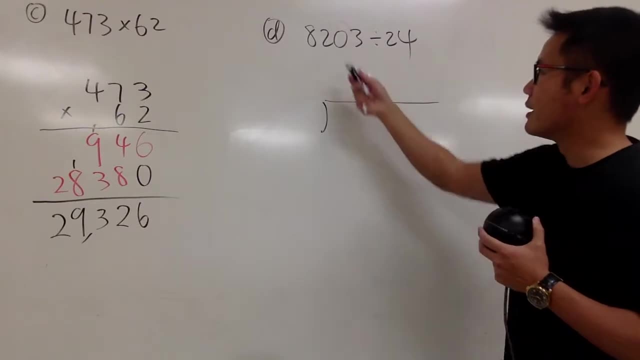 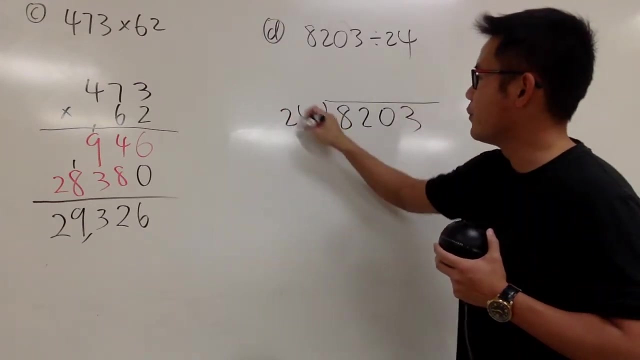 2,000,, sorry, 29,326.. Now, moving on to division. This is how we do. it Start with a long division bar And we put the first number inside- 8,203, like this, And then we have the 24 on the outside. 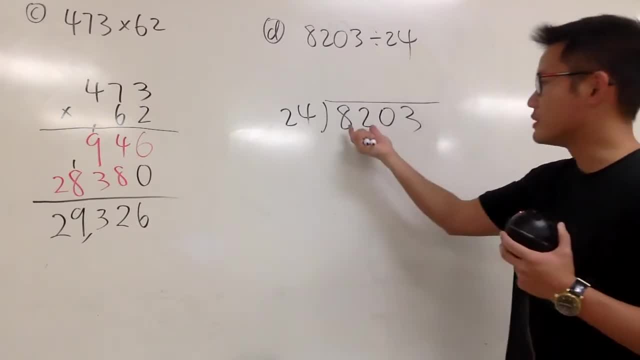 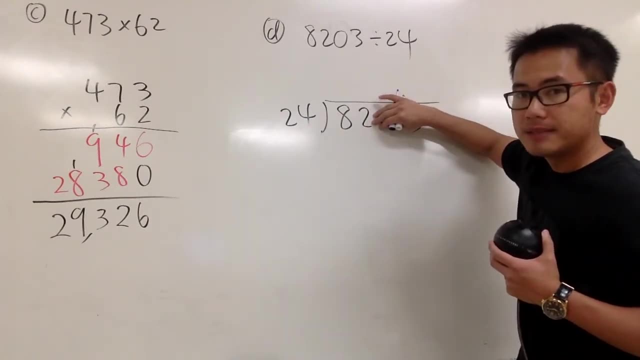 And because we have two digits outside, let's compare with the first two digits, Which is right here as well. We are going to ask ourselves: 24 goes into 82. how many times? Well, we know, 24 times 2 is 48.. 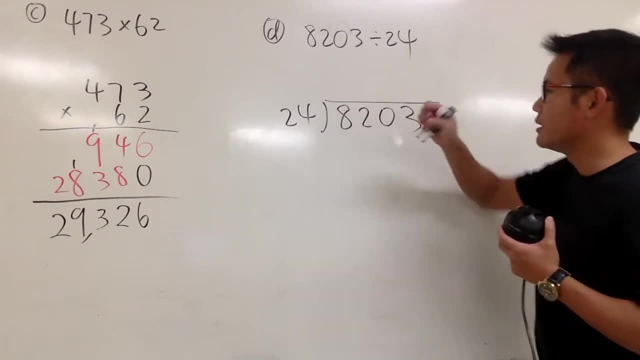 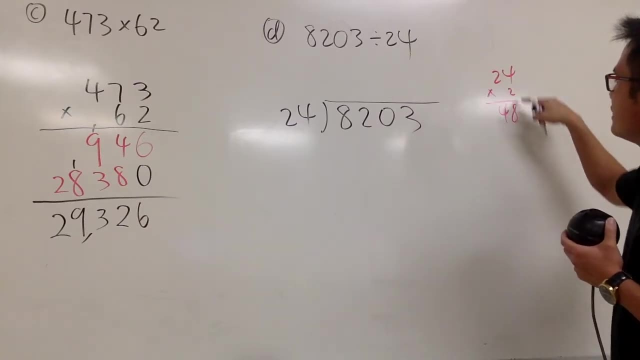 24 times 3 is 72. Right, So let me write it down for you guys. Let's put down 24 times 2.. We know this is 8.. This is 4. So 48, right. 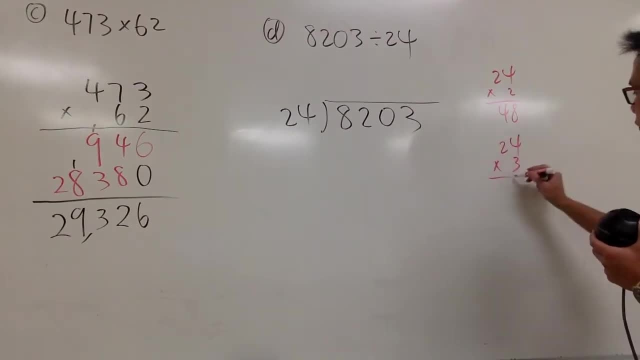 And then, if we do 24 times 3,, 3 times 4 is 12,, like this, And then 3 times 2 is 6.. Plus 1 is 72.. And that's actually enough, Because if you have one more, 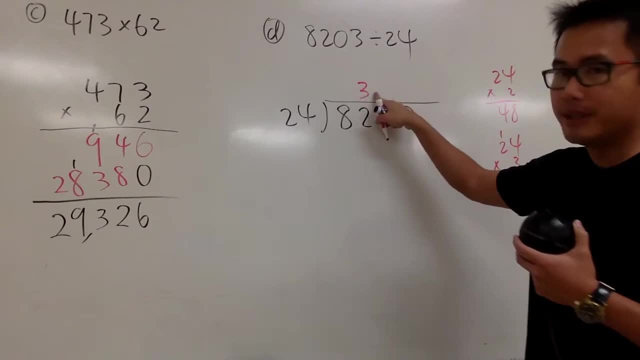 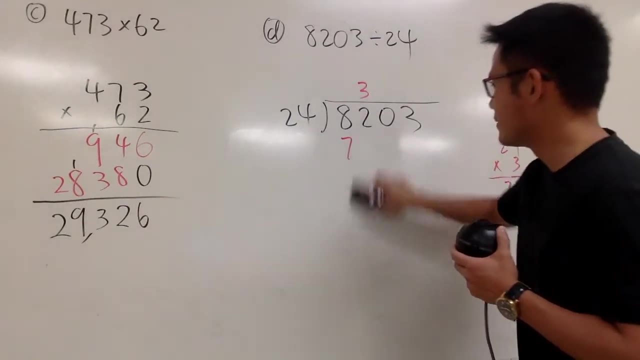 it's going to go over. So that's no good. So we will have 3.. Now, 3 times 24, we get a 78.. Because we get a 72, because we did it right here, Right. 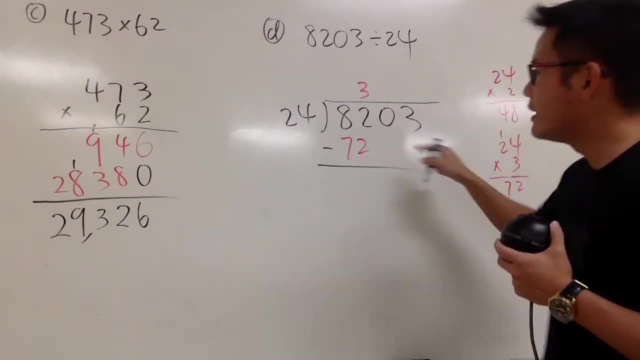 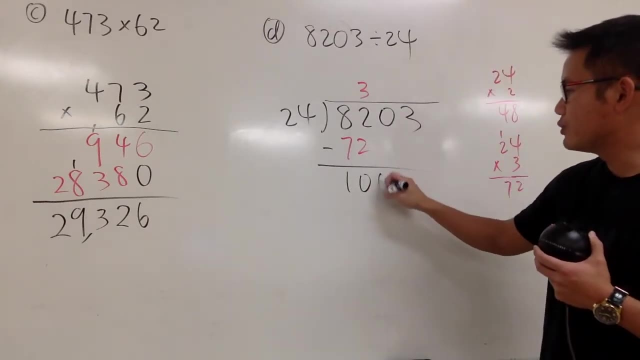 We did it right here. And then we continue by subtracting, And 82 minus 72, we get 10.. And then you bring down the next number, which is 0. And you are going to ask yourself: 24 goes into 100. now, 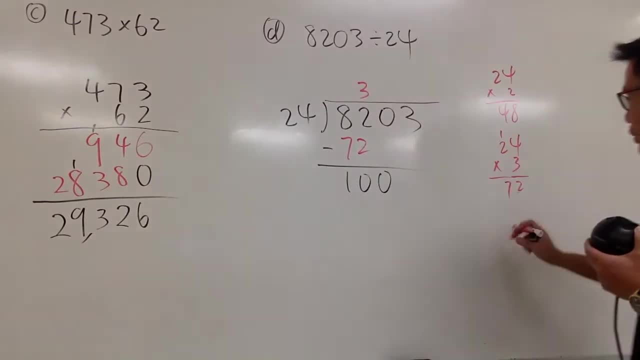 how many times? And the answer to that is 4.. I'll show you: 24 times 4.. 4 times 4 is 16.. And then 4 times 2 is 8.. Plus 1 is 9.. 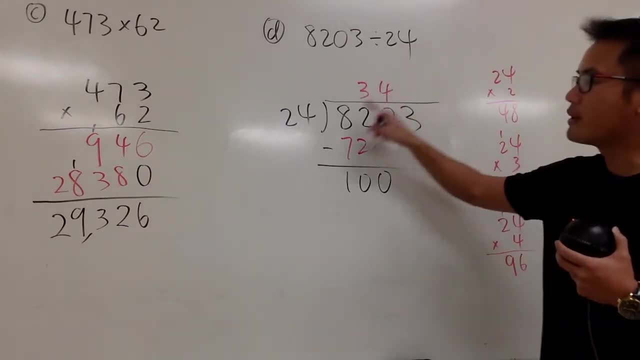 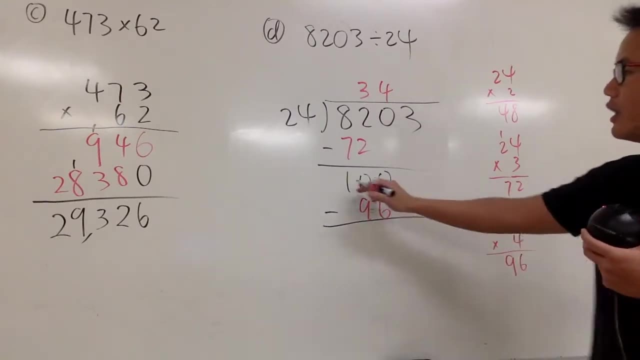 So if I put down 4 here 4 times 24, we get 96. And then we can proceed with: subtract 100 minus 96, we get 4.. And then we bring down the 3 right here. 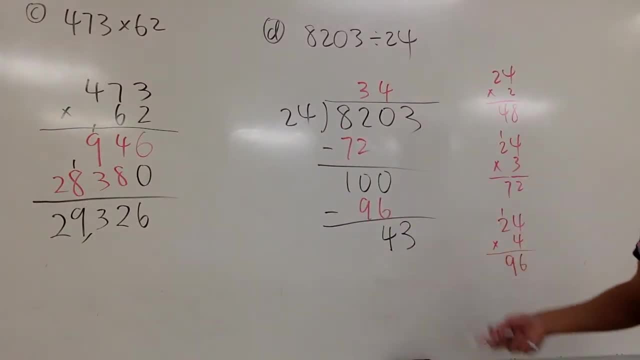 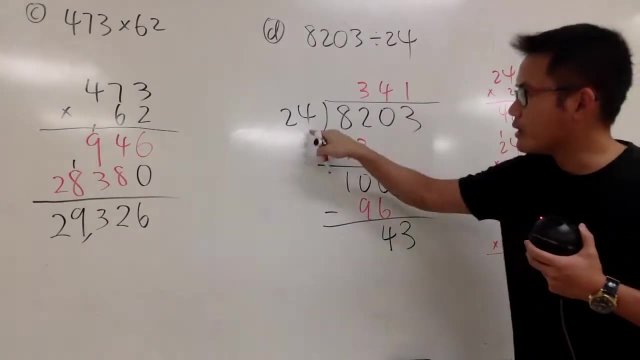 And now 24 goes into 43. how many times? Only 1 time, Because when you have 2, this is 48, right, So we'll just have 1 time. 1 times 24, we get 24.. 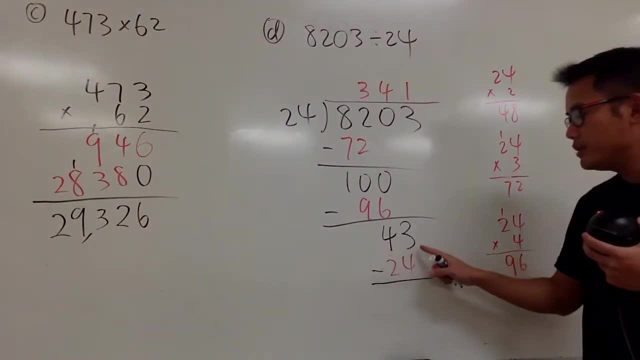 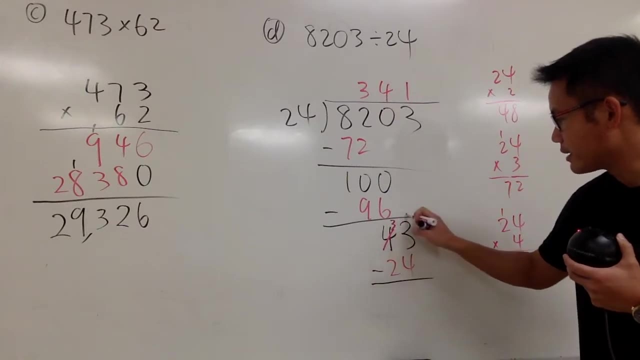 And then we'll subtract 43 minus 28.. So we are going to do this right. 3 minus 4, I have to borrow- So this becomes a 3.. This becomes a 13.. 13 minus 4, we get 8.. 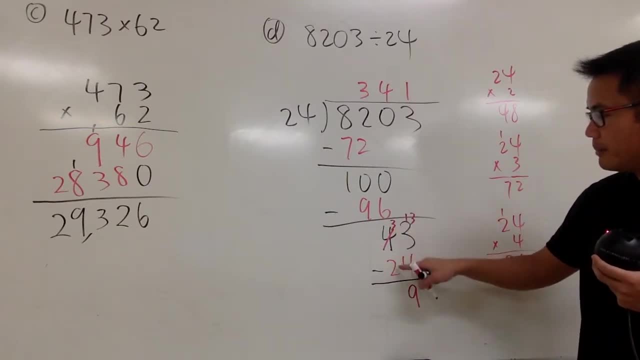 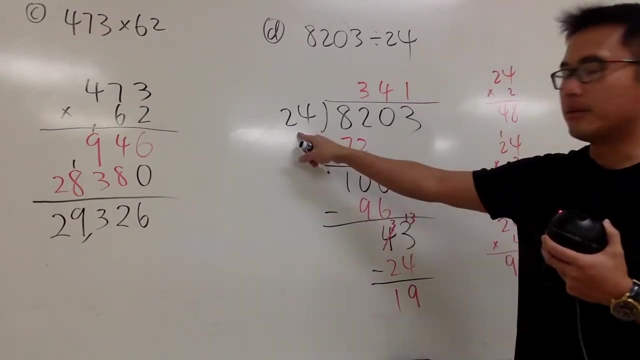 3 minus 4, we get 9.. And then 3 minus 2, we get 1.. And that's the remainder. And you just have to be sure the remainder is smaller than this number and we are done right. 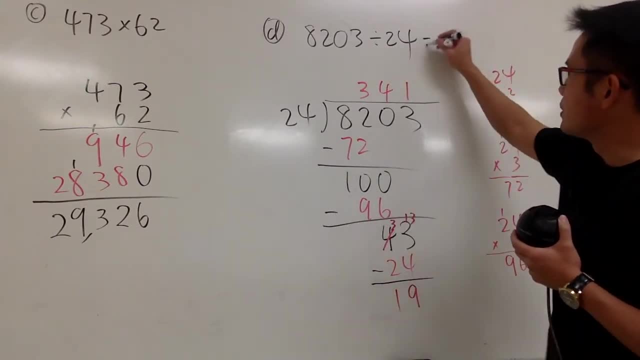 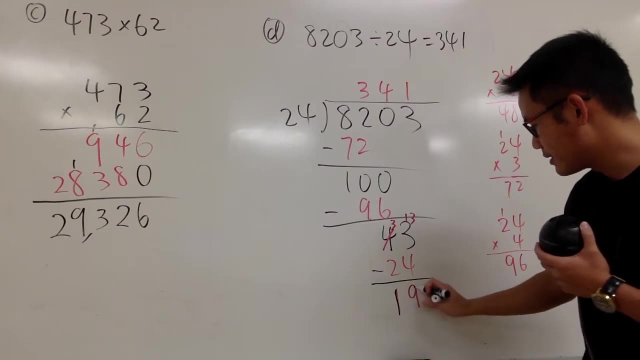 And this is how you write down the answer for diffusion. You write down the answer as- let me put it down here: 341, right here, with the remainder. I should put this down in black- with the remainder 19.. 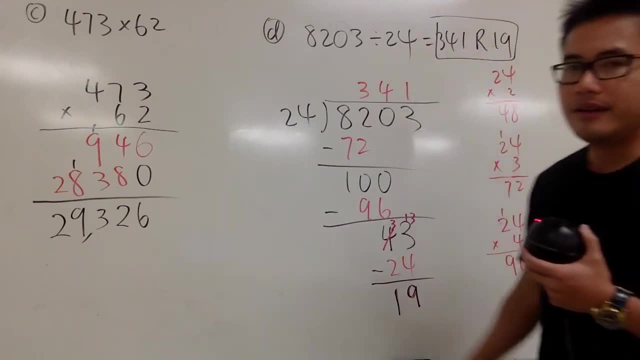 So put down R 19,. like this And earlier this answer was this right here. So yeah, that's it.